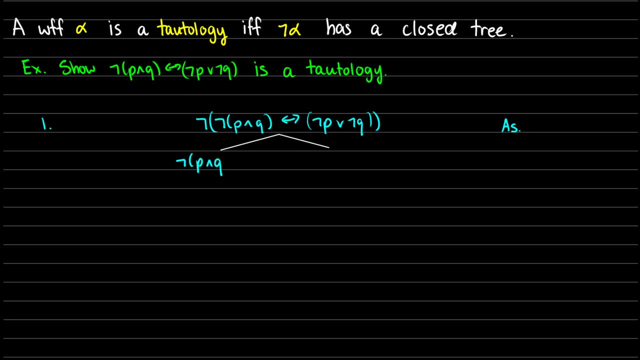 So we're going to get not P and Q as our first thing, and we're going to get not P or not Q as our second. So, in other words, the left side is true, the right side is false, And on our other branching path we'll get the opposite. 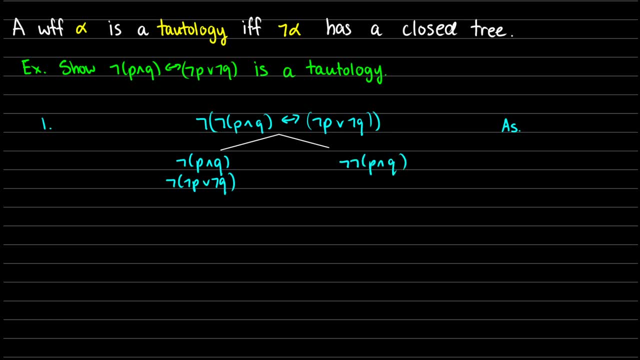 So we're going to get not- not P and Q- by taking the left side to be false, and we'll get not P or not Q by taking the right-hand side to be true. So these are our two situations. So this is line 2 and line 3, and these both come from 1,. 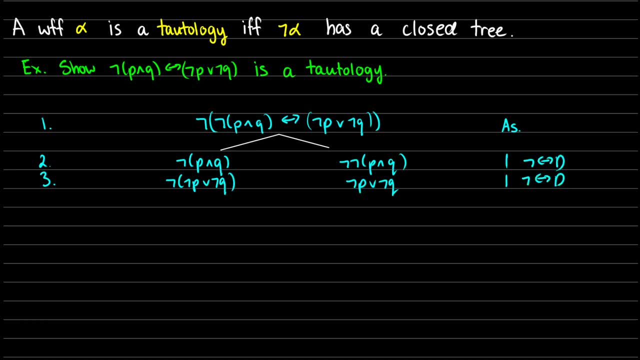 and this is not biconditional decomposition. Okay, I have a choice what I want to do here. Okay, What I'll do, just to make it simple, after we check one off because we're done with it, we'll go to line 4, and I'm just going to get rid of the not, not P and Q on the right. 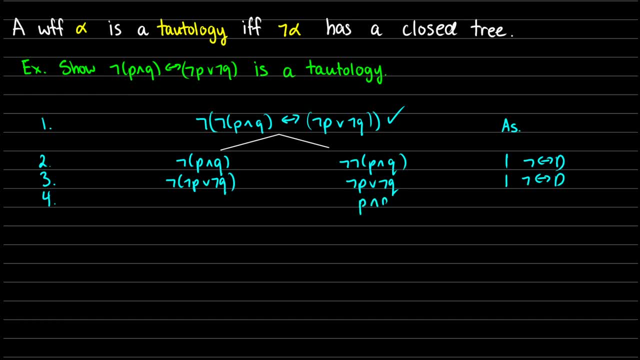 So we'll do double negation to get rid of those negations. So we'll be left with P and Q. Check that off. That comes from line 2, and that's double negation. Now, since I have P and Q, why not? 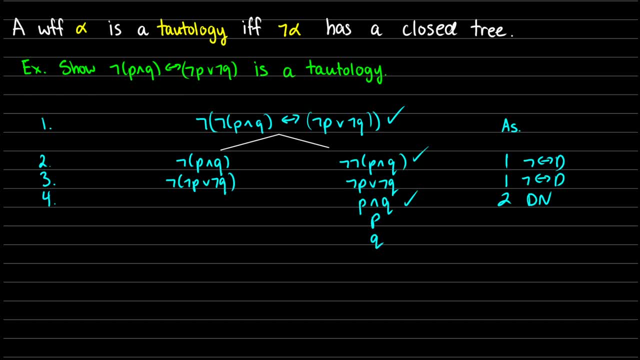 Let's just get rid of the and so we know we get P and we get Q. That'll be line 5 and 6.. So from line 4, we're doing and decomposition. Well, at this point on the right side, we only have one thing left to do. 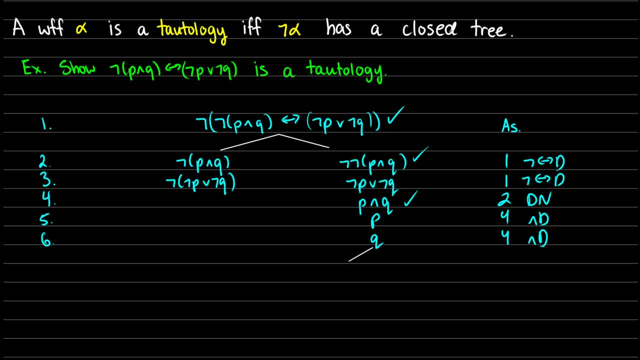 which is to take the branching paths with not P or not Q. So let's do or decomposition, which will give us not P, not Q. So this is line 7.. This comes from line 3, and this is: or decomposition, 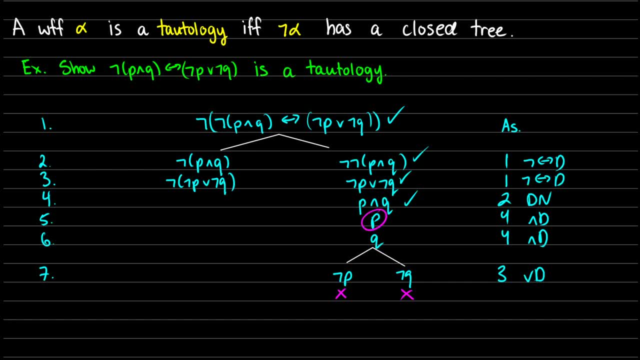 At this point our right branch is closed because we have P and we have not P, which closes that branch, and we have not Q and we have Q, which closes our right branch. So that side's done. Now I'm realizing I'm going to need a little bit more space on here. 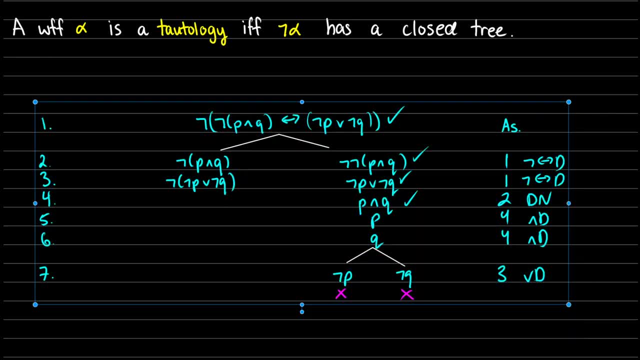 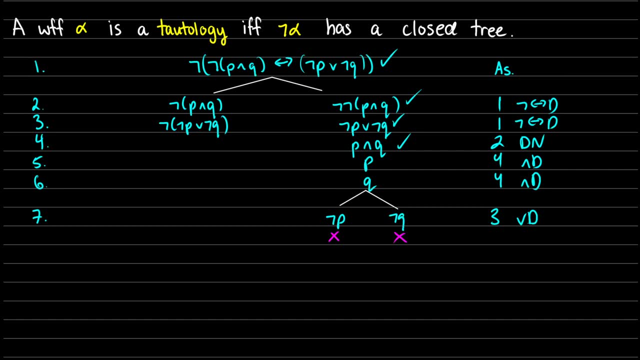 so what I'm going to do is I'm going to get rid of the question and I'm going to move this up, so that way we do not have to scroll onto another page. Okay, So our right side's done. Now we have to do our left side. 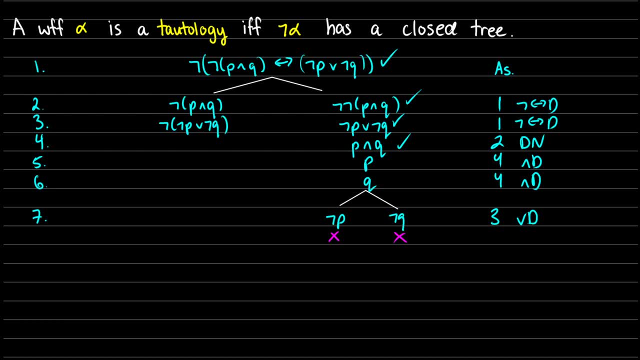 We have a choice here. We can do not P and Q first, or we can do not not P or not Q first. Now, if you remember, if we have not P or Q being true, this means that P or Q is false. 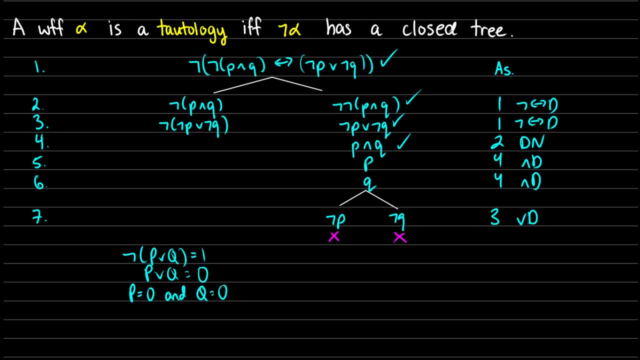 which means that P is false and Q is false in order for that to be true, which is the same thing as saying: not P and not Q are both true. So, in other words, we don't have to take branching paths if we do not, or decomposition first. 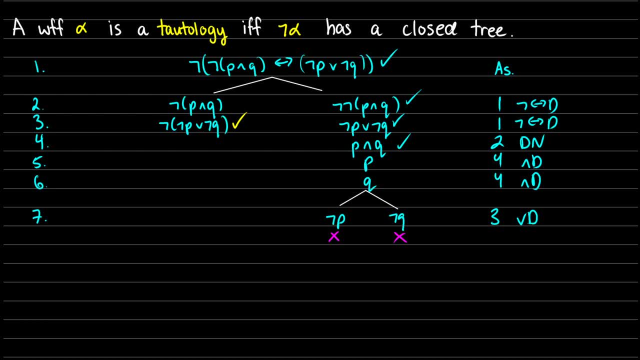 So let's take care of that. In fact, I'll do it in yellow, Why not? So in line 8 and line 9, we're going to get not, not P and not not Q, But this comes from line 3 on the left branch, and this is not or decomposition. 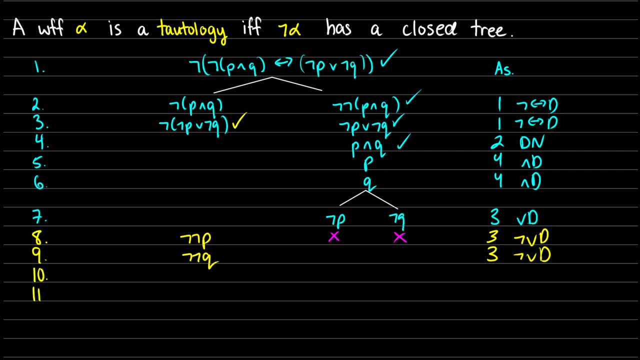 So hopefully by now you're more comfortable with that rule At this point. in lines 10 and 11, let's get rid of those double negations there, since those don't help us very much. So we'll get P and Q. 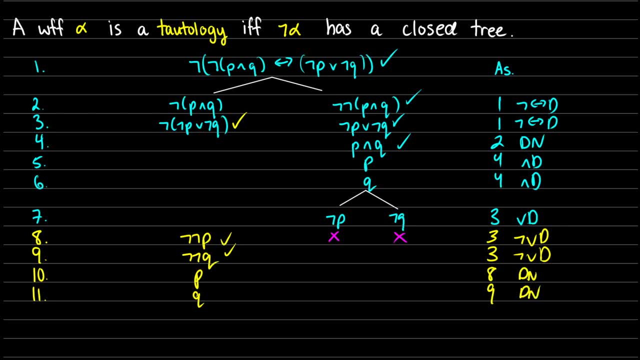 So from line 8 and line 9, this is just double negation. Okay, there's only one more thing left to do in our tree. Let's do it in green. We're going to decompose, not P and Q, So this is going to give us two branching paths. 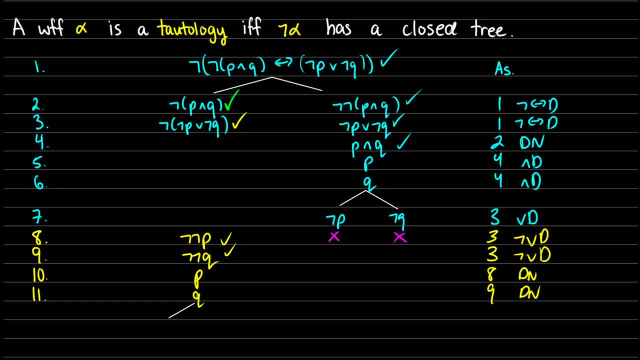 On one of the sides of this path we're going to get that not P is true, And on the other side we're going to get that not Q is true. So again from that reasoning we know not P and Q is true if P and Q is false. 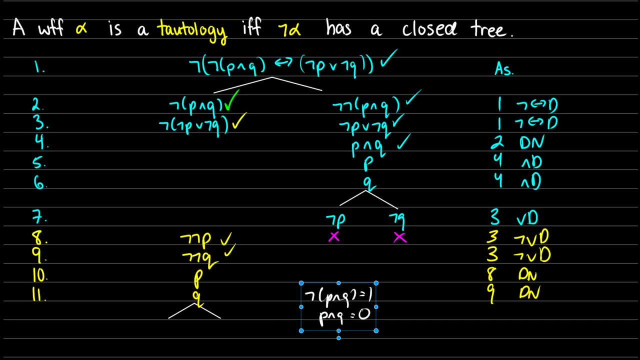 which means either P is false or Q is false, which means not P is true or not Q is true. So that's going to give us not P on the left, not Q on the right. This is line 12. And this is justified from line 2, which is not and decomposition. 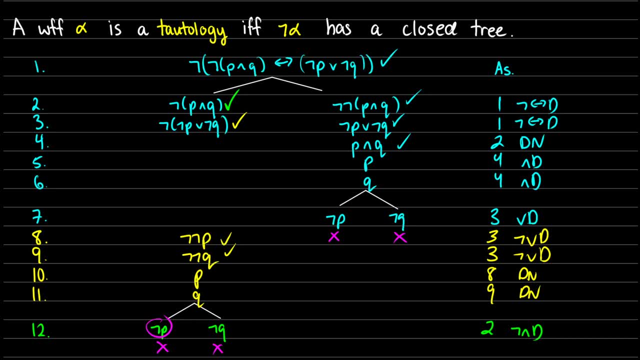 And at this point both of these branches close because we have not P and we have P and we have not Q and we have Q, which gives us a contradiction. So we just have enough room on this page in order to determine that. 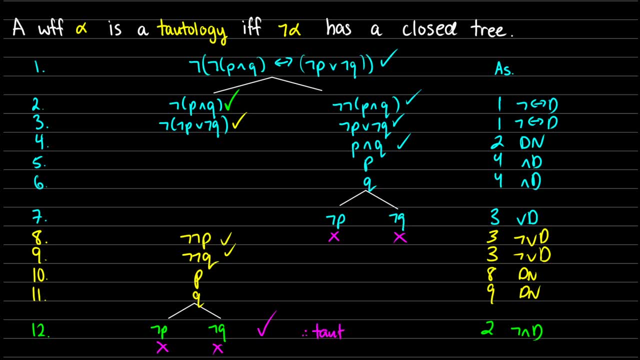 yes, all of these branches close. Therefore, what we looked at is a tautology. Now, one thing you can do in a tree if you want one gap is you can put a little line there just to symbolize that those things are connected. 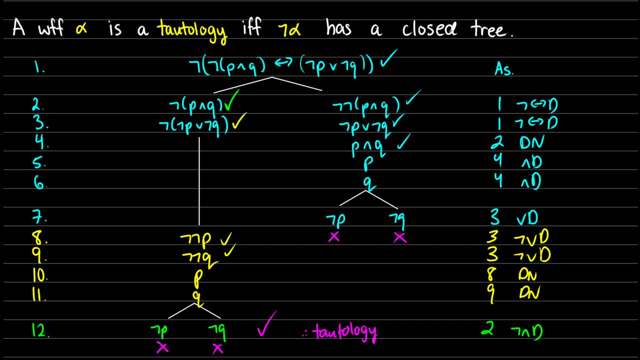 It looks a little bit nicer, especially when you go from one branch to the other. but that is totally up to you if you want to do that or not. Anyways, that's a tautology. The important part with tautologies is how we start. 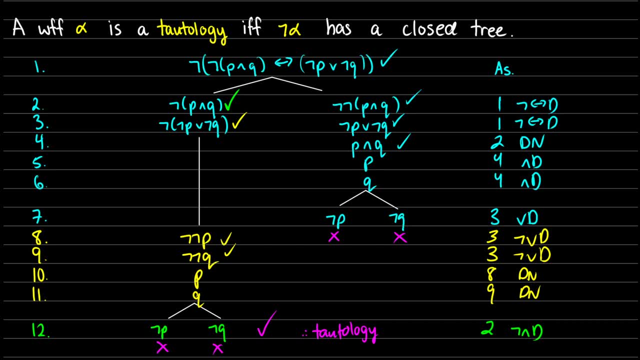 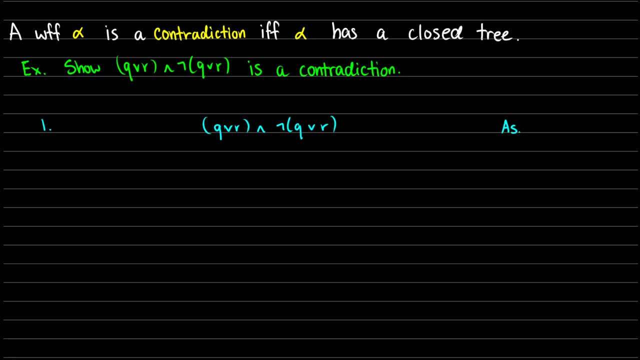 We have to start by negating it and then showing that the non-tautological assumption does not hold With a contradiction. it's quite straightforward: If something is a contradiction, then the tree should close. So if we want to prove that alpha is a contradiction, 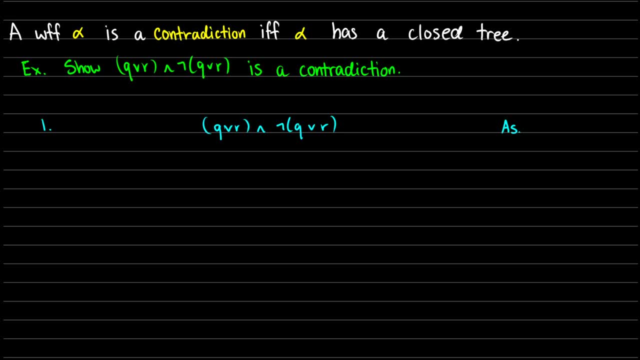 we just have to work with alpha itself and close all the branches. So I want to show that QR and not QR is a contradiction, So let's work with that, Okay, well, we have AND in our first line. So this makes things really easy because we can just break one apart. 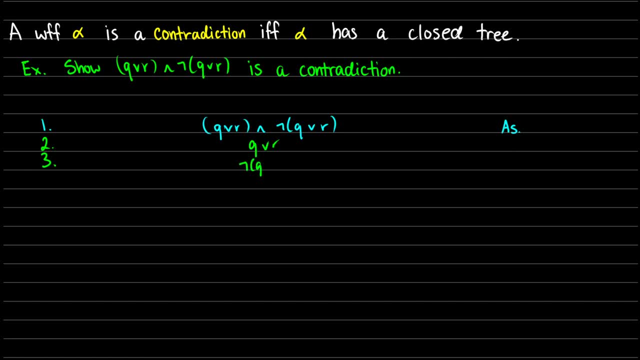 So we know that QR is true and we know that not QR is true. So these both come from line one, and this is: AND decomposition Done. Okay, next step, Let's do not QR, for the same reason as before. We know, then, that not Q is going to be true and not R is going to be true. 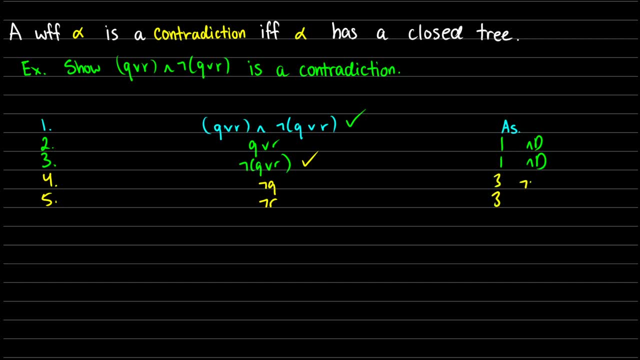 So that's line four and five. This comes from three and this is not OR decomposition. Remember, we want to do AND decomposition and not OR decomposition as soon as we can, because we don't get our branching paths here Now. the only thing left to do is to do QR. 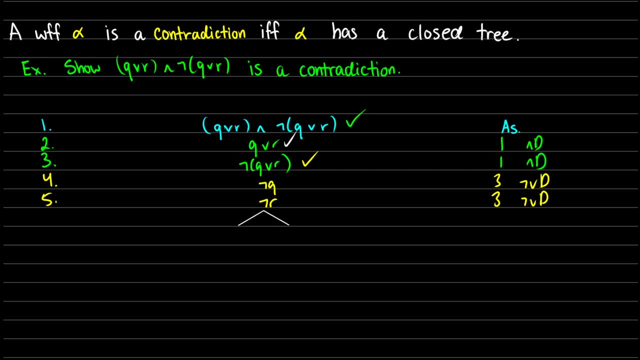 So we're going to get some branching paths here. We're going to get one case where Q is true, one case where R is true. So this is line six. This comes from two OR decomposition, and we'll find that both of these close. 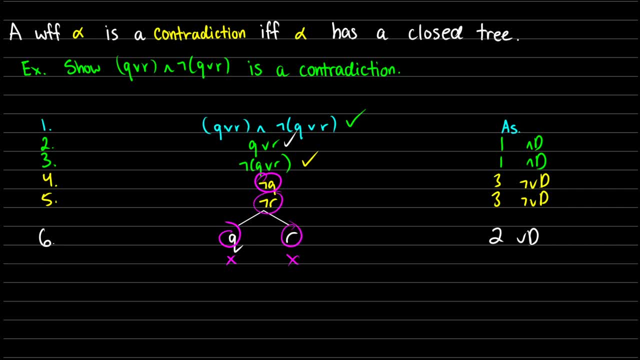 because we have Q not Q, R not R, So we get a contradiction on both sides. It closes: Okay, easy. Therefore, we know that this is a contradiction, because there's no way that we can make this tree true. 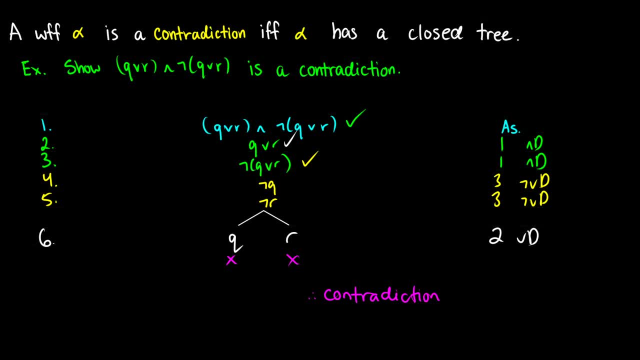 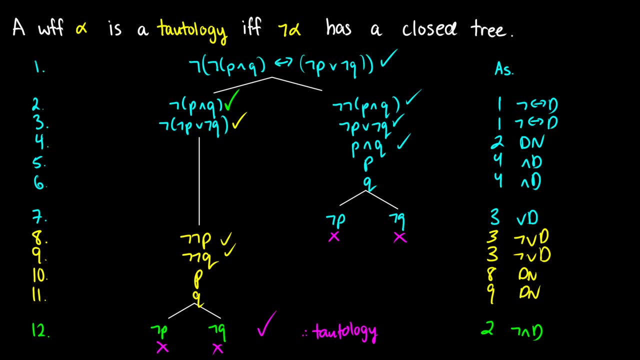 So if I take off the lines here, we can see it in all of its beautiful glory. In fact, let's take a look at the previous tree without the lines on the page so we can see it in its beautiful glory. Everything just looks nicer without lines on the page. 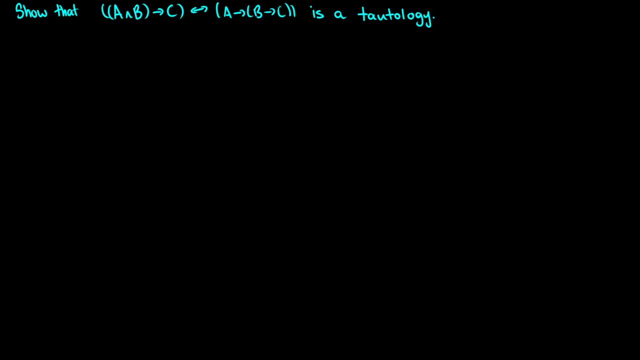 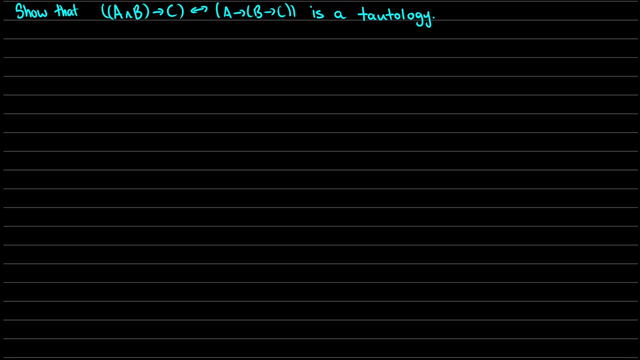 I don't know why that is, It's just a fact of life. Anyways, one more practice question. Let's show that this monster is a tautology. So our first step is setting it up. We want to prove that this beast is a tautology. 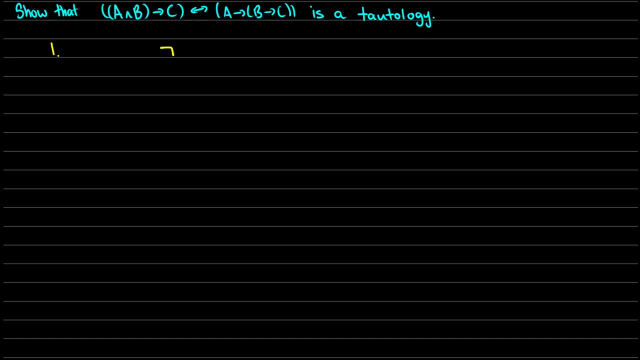 So that's our alpha. What we have to do is we have to negate this. We have to take the negation of all these things, which means we're going to have a lot of brackets here. What we're going to have is we're going to have 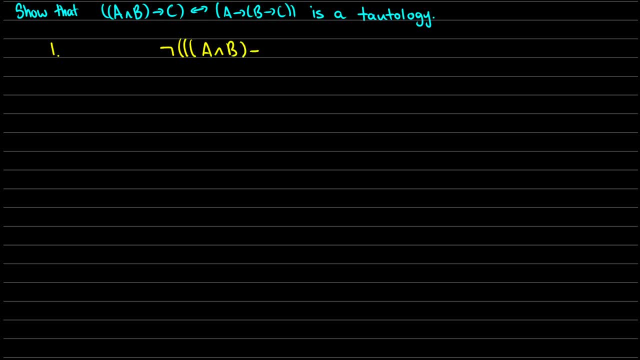 not. if A and B, then C is the same thing as A arrow B, arrow C. Okay, and this is our assumption. So we're going to have branching paths here and this might get a little bit long. Hopefully we can put this all on one page. 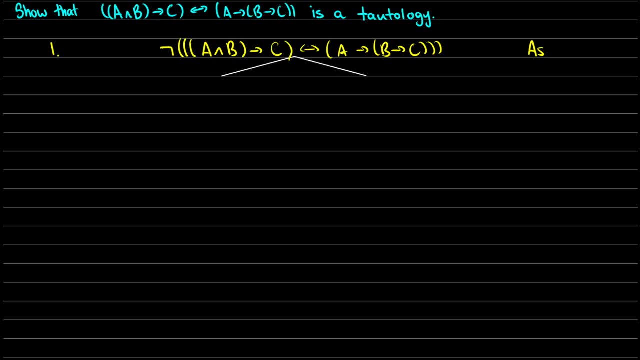 So on our left side, remember it's going to be either one of those is true and one of those is false, or vice versa. So on our left side, let's just assume that the left is false. So we'll get not A and B arrow C. 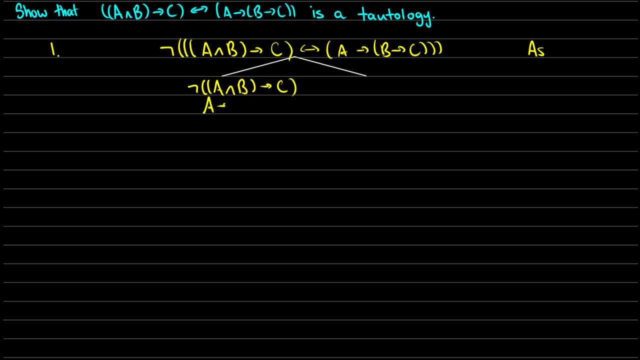 And that means we'll also get A arrow B arrow C, And on the right hand side, we'll assume that A and B arrow C is true And we'll then assume that not A arrow B arrow C is false. Okay, so this is line two and line three. 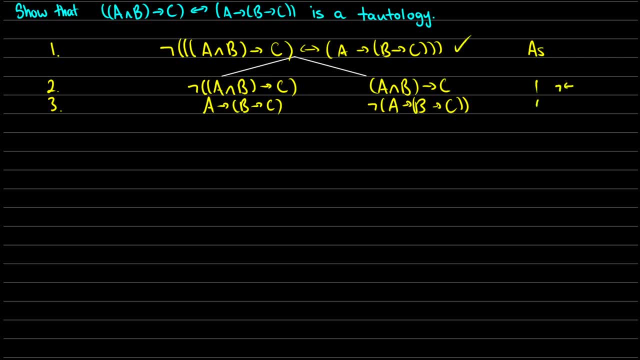 That comes from line one, And this is our not biconditional decomposition. Okay, I can already tell this is going to be a bit of a gross proof, But the nice thing is: first, we have not arrow, So remember, if we have not A, arrow B 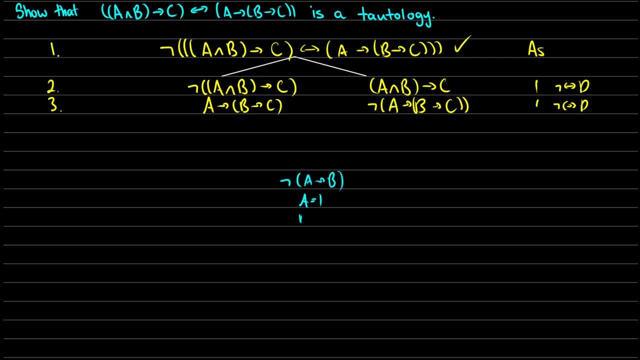 what we're saying is: when is this not true? It's not true when A is true and B is false, which is the same thing as saying that not B is true. So we can break our not arrows into the antecedent being true. 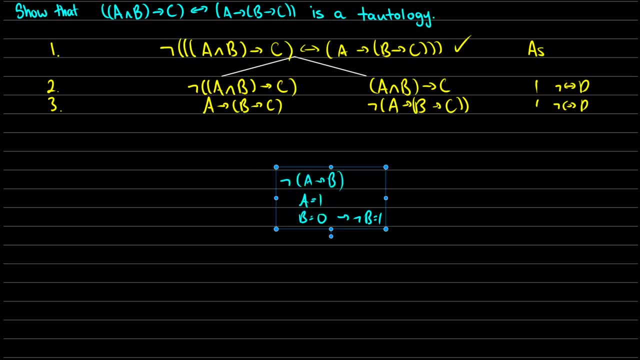 and the consequent being false. So what this means is that on line four and line five we could say: check off two, for example here. So in this case we'll get that A and B is true And we'll get that not C is true. 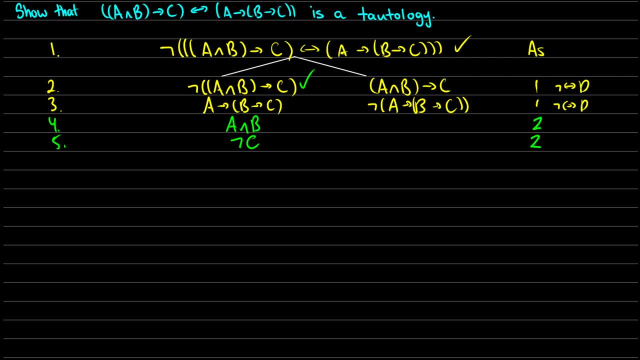 Okay, so this comes from line two And this is not arrow decomposition. I can actually do this on the right side too, So that'll come from line three. It's different. I'll justify it on the right, but it's the same step. 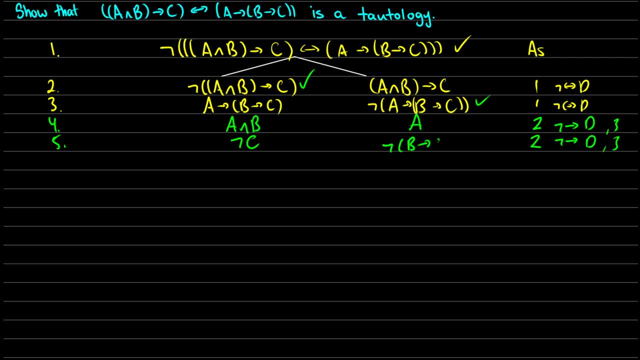 So we're going to get A is true And we're going to get not B arrow. C is true. Okay, well, on the right side, this is actually nice because we have another case of the not arrow, So we're going to get that B is true. 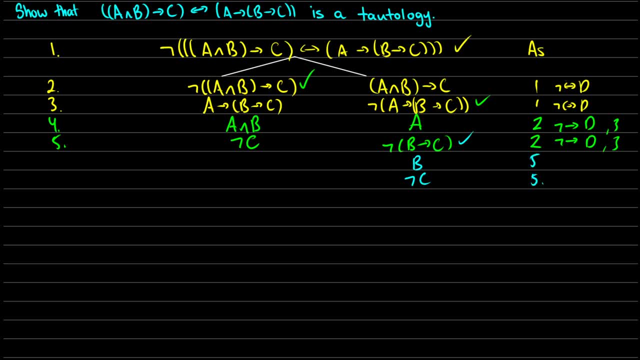 And we're going to get that. not C is true there. So that's going to come from line five And it's the same idea. It's not arrow decomposition. Okay, I have nothing yet that is wrong on the right side. There's no contradictions yet, but we're pretty much one step there. 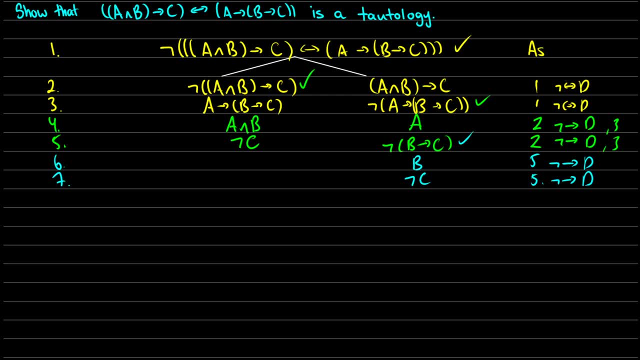 So why not just finish it? Okay, so we need to do A and B arrow C, which means we're going to have branching paths. Either the antecedent is false or the consequent is true, So we're going to have one case. 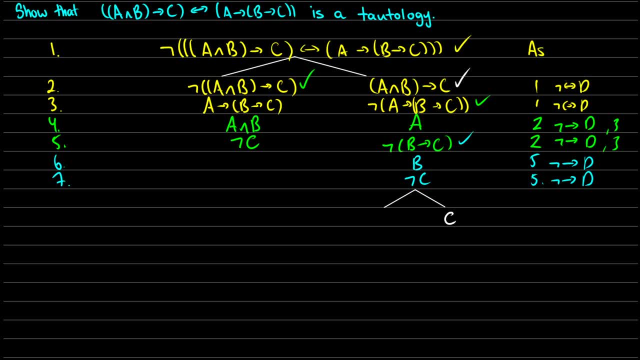 Let's do this in white, where C is true, And we'll have one case where we have not A and B, So the antecedent is false. Now our C branch. we can finish, because we see that we have C and we have not C. 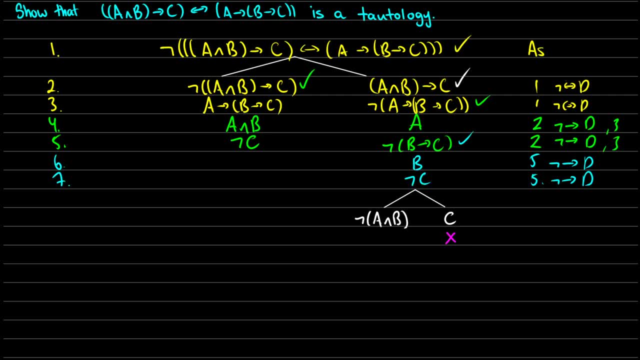 So we have a contradiction there. that's closed, So we should label this before we go on. This is eight. This comes from line two. This is arrow decomposition. We're going to have some more branching paths here, So not A and B is going to give us either not A or not B. 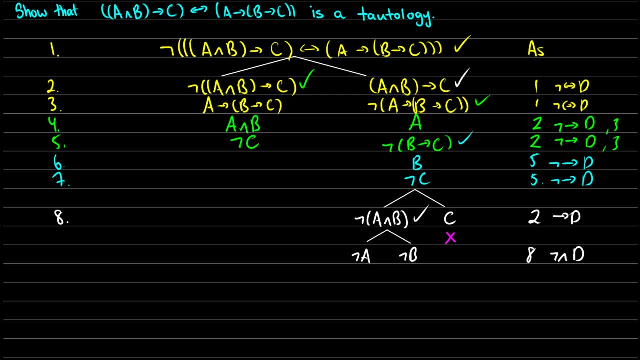 So that comes from line eight And this is not. and decomposition on line nine. Okay, At this point too, we can then close off not A and not B, Because we have A and we have not A, And we have B and we have not B. 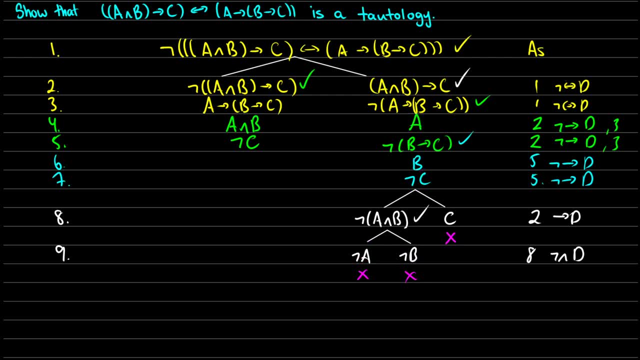 So we get contradictions there. Okay, so our one side is now completely done. We can now focus on the left side. So we have line ten down here. Let's just make a little path here so we know that we're continuing, And for convenience, because we have A and B and we have not C. 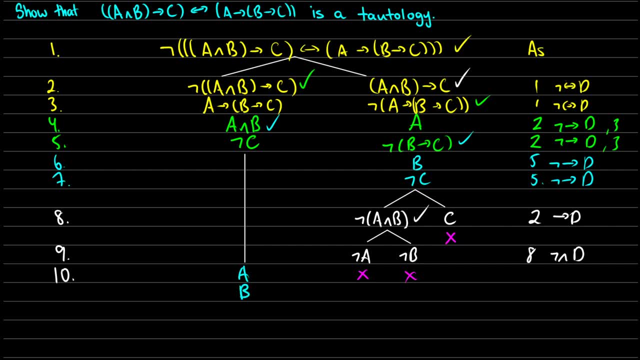 let's just get rid of this. A and B. Let's break this into components, So we're going to be left with A- B. So this comes from line four And this is and decomposition. Okay, so we still have just one thing left over here. 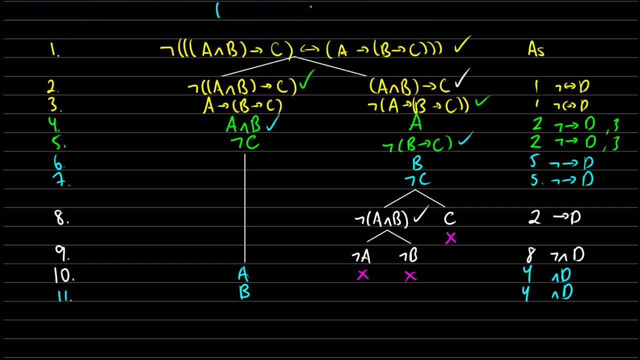 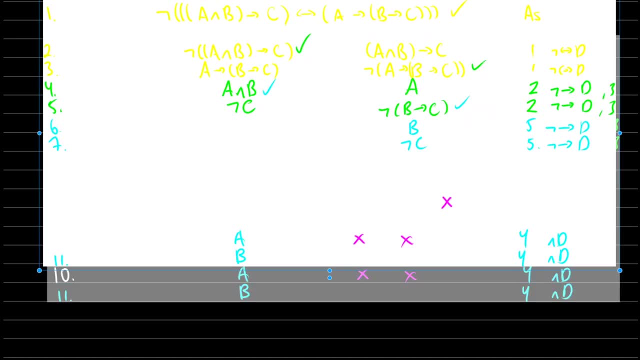 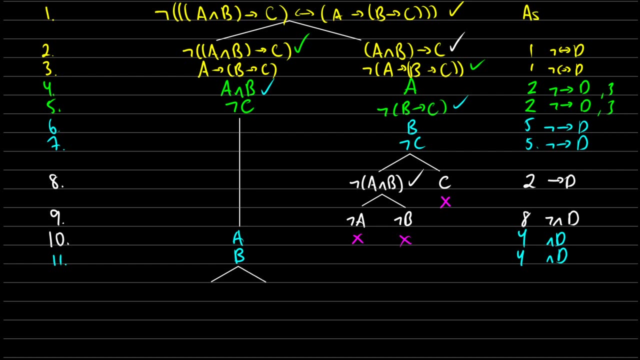 In fact, what I need to do is I need to get rid of this question at the top And I think I need to start moving things up so we can keep everything on the page. Okay, so we're going to get branching paths because we have A arrow B, arrow C. 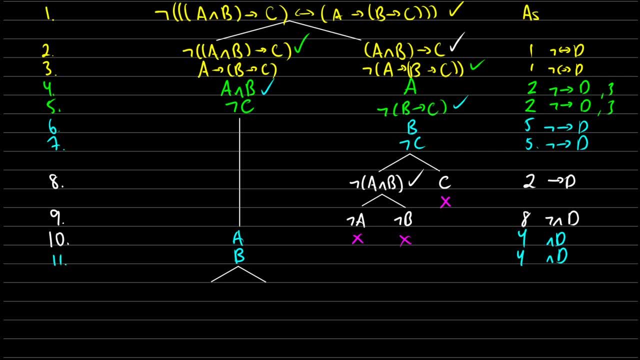 Which means either the antecedent is false or the consequent is true. So when we check off from line three here, we're going to get either not A or we're going to get B. arrow C. This is line twelve. This comes from line three. 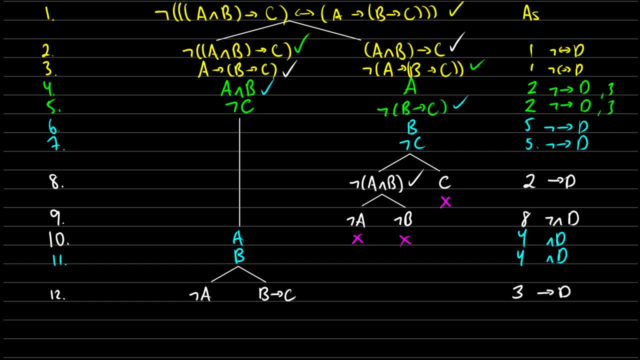 And this is arrow decomposition. Okay, our not A is now going to close because we have not A and A. So we get a contradiction. Our last step will be another disjunction here with B arrow C, So this will break off into two paths. 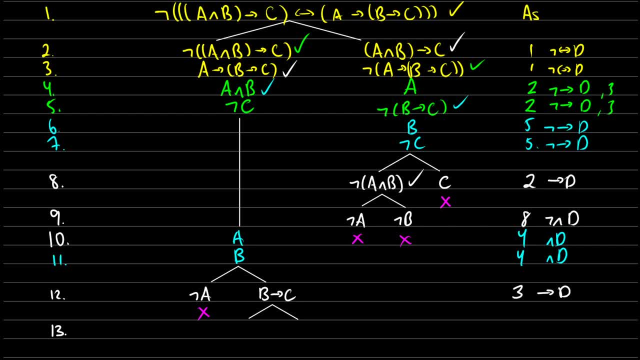 By the conditional, either B will be false or C will be true, Which means we're going to get either not B or we'll get C. So that one's done. This comes from twelve, And that's arrow decomposition. At this point we can now close these branches, because we get not B and B. 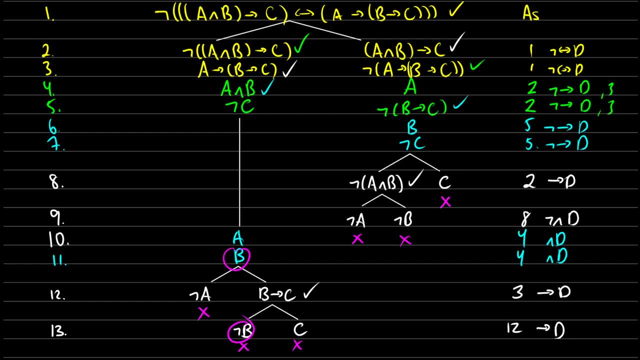 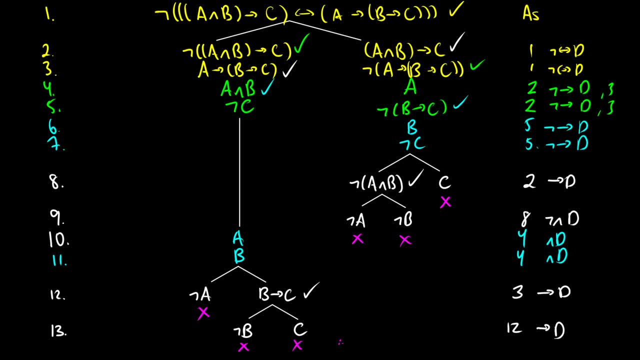 That's a contradiction. And we get not C and C. That's a contradiction. Therefore, everything closes. So we know that this is therefore a tautology, And it's a tautology because the negation arrow of original sentence closed. 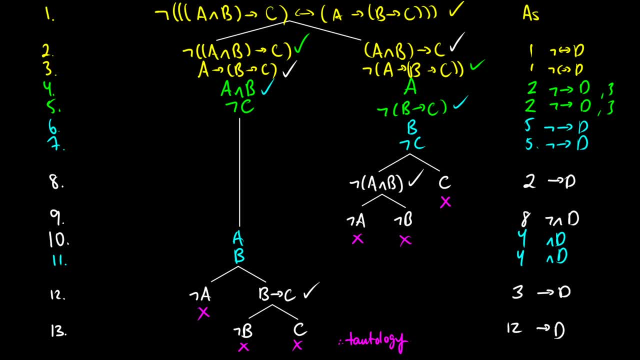 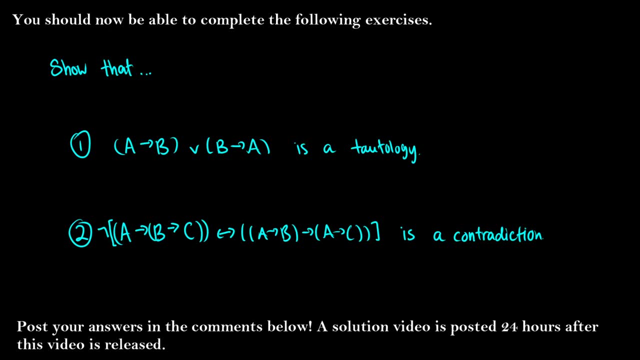 So that's it for tautologies and contradictions. At this point you should be able to complete the following exercises. So I want you to try with your own truth tree to see whether one is a tautology and two is a contradiction. 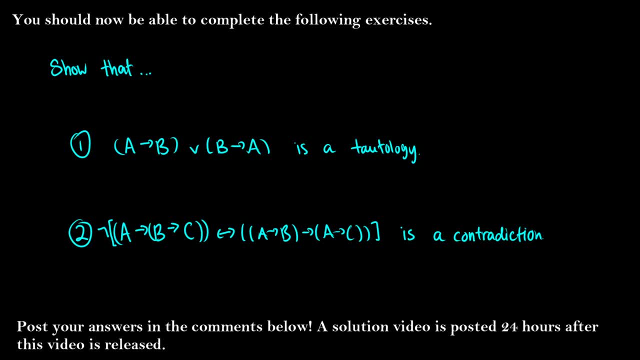 Somehow you can post your answers in the comments below. Go for it, But I think it's going to be incredibly difficult to do with truth trees. Anyways, if you have any questions, post them in the comments below And I'll do my best to help you. one again. Thank you.